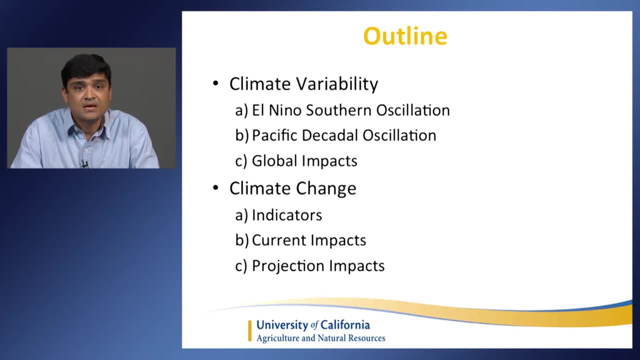 especially for California, And I'll give you some examples of very well-known phenomena called El Nino-Southern Oscillation, Pacific Decade, El Nino, El Nino-Southern Oscillations and et cetera, and then how they might impact climate across the globe. 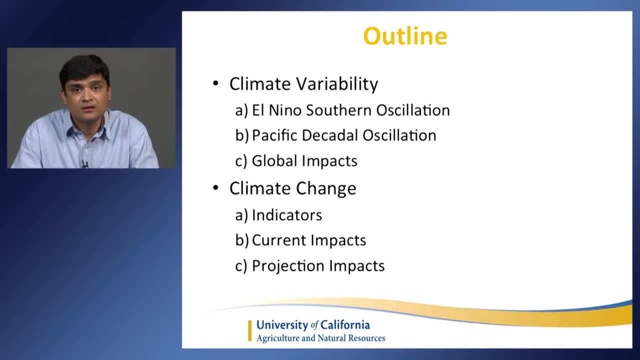 including here in United States, And then I'll move into and talk about climate change indicators, what we have seen over the past hundred years and what we might expect in future in terms of climate projections, and what are the projected impacts. So climate variability. 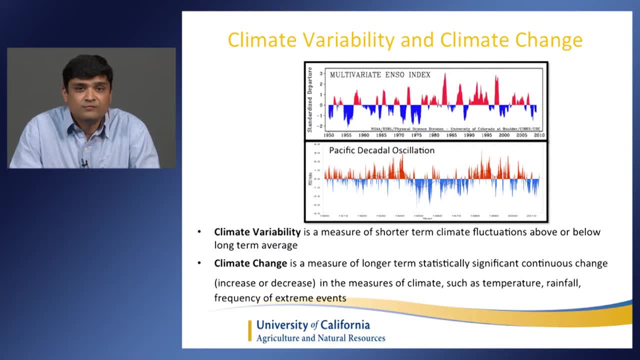 versus climate change. By definition, when we mention about climate variability, it's a measure of short-term climate fluctuations above or below their long-term averages. So if you look at this top figure, it says multivariate ENSO index. This is one of many indices that are created or developed. 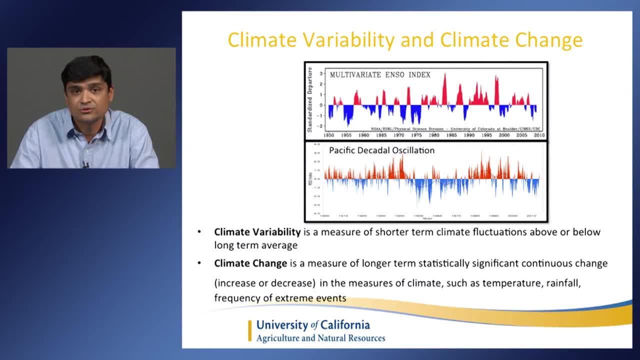 in terms of identifying El Nino-Southern Oscillation patterns And, as you can see, these oscillations in the time series range anywhere from six to 18 months, So it's a rather short-term fluctuations And the way El Nino, La Ninos are defined. 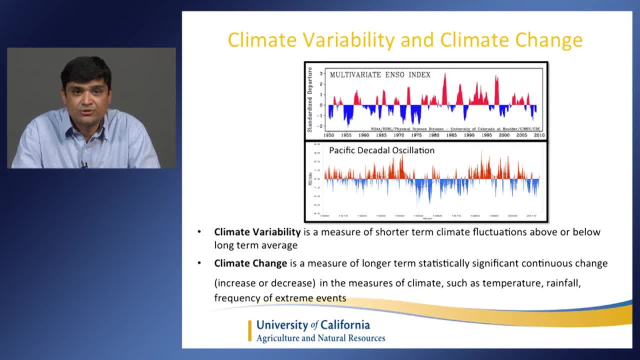 is when sea surface temperature in equatorial Pacific region is about normal for a certain period of time. That phase is called El Nino. What we've seen this year is one of the strongest, the most significant and the most significant change in climate change. 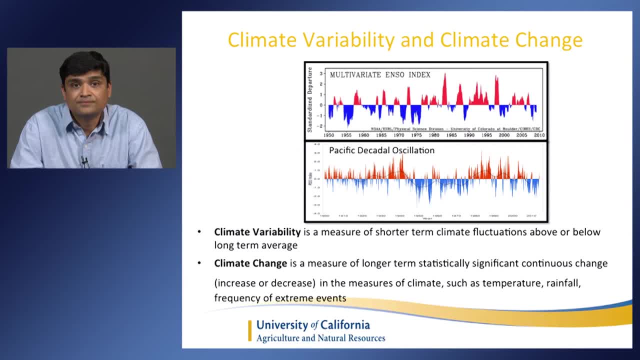 in the world. This is the strongest El Nino on record And, as opposed to that when sea surface temperature in that equatorial Pacific region, it's also called Nino 3.4.. In that region, when sea surface temperature is below normal for longer period of time. 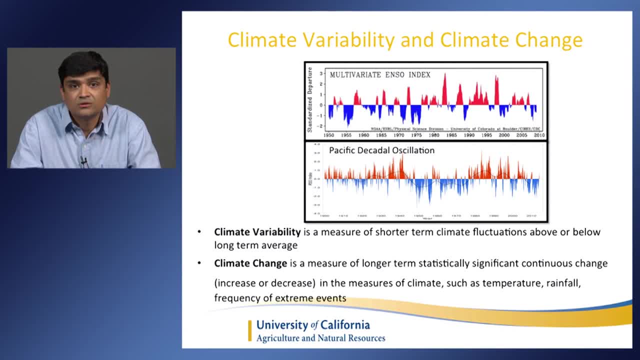 that phenomenon is called La Nina And together it's called El Nino-Southern Oscillations. But when we are not even in El Nino or La Nina phase, the third phase is called neutral, where sea surface temperatures are neither warmer nor cooler. 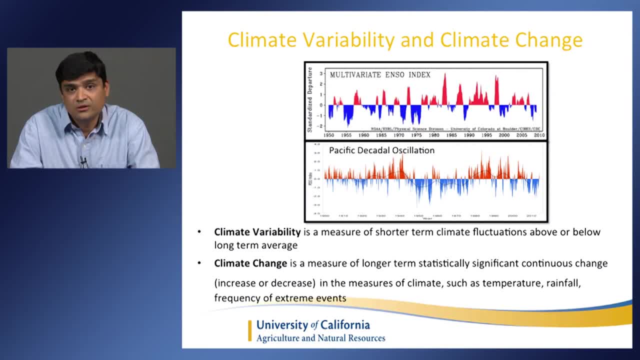 So when you look at El Nino or La Nina impacts on climate across the globe. it varies significantly, but their timeframe is rather short-term. There is another oscillation that I wanted to mention here is called Pacific Decadal Oscillation. It's if you look at this time series. 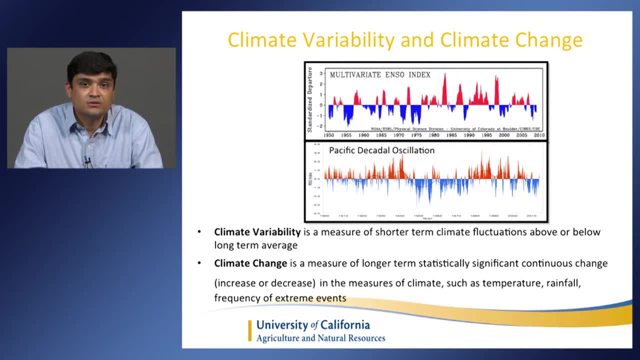 their oscillation range anywhere from, you know, from the Pacific Decadal Oscillation to the Pacific Decadal Oscillation, 10 to 20 years, So it's a rather longer term oscillation And with respect to their warmer or cooler conditions, 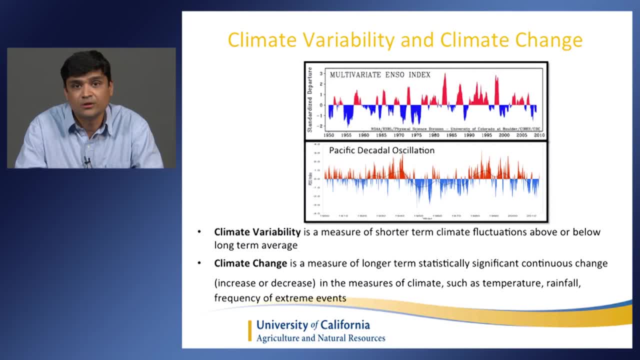 they can impact climate significantly across the globe, including here in United States. The other thing I wanted to point out, especially in the climate variability section, is, you know, as opposed to El Nino, especially in the Pacific Decadal Oscillation. 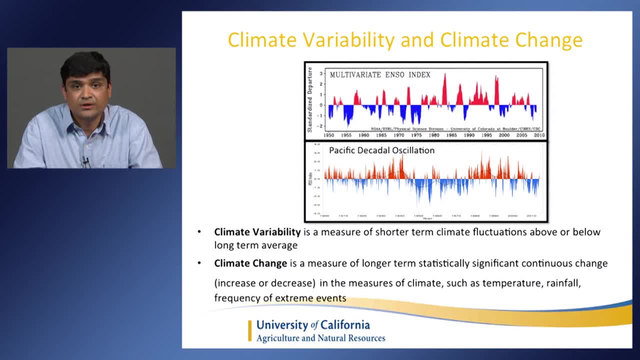 in their warmer phase. the coastal area in United States, all the way from Alaska to the equator, are experiencing warmer than normal sea surface temperature, But at the same time it's cooler than normal in a tropical Pacific region And in a cooler phase of Pacific Decadal Oscillation. 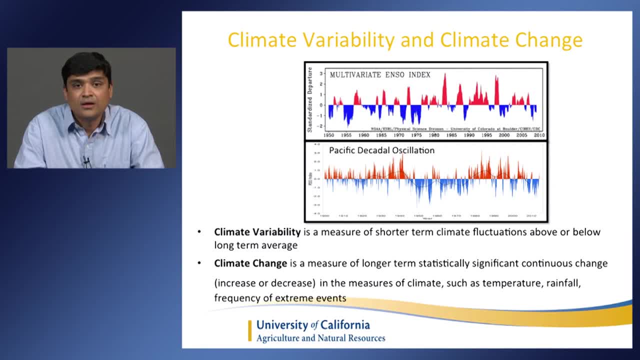 whole process is the other way around And when both these phases for El Nino and La Nina and the Pacific Decadal Oscillation, if they are in a similar phases like positive or negative, or warmer or cooler, that can signify impacts of climate. 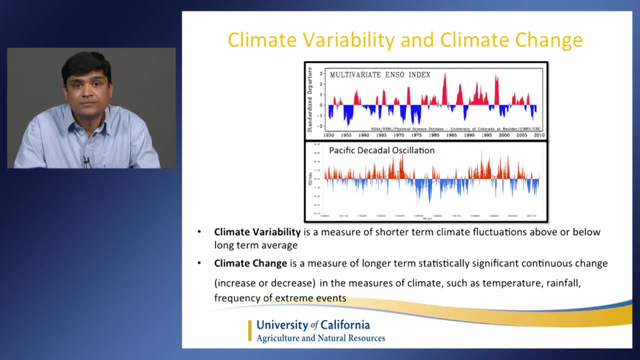 or it can vary climate across the globe quite significantly, as opposed to one being on the positive side, the second being on the negative side. So, and these are just two examples of large-scale tele-connection techniques that can be used in the climate variability section. 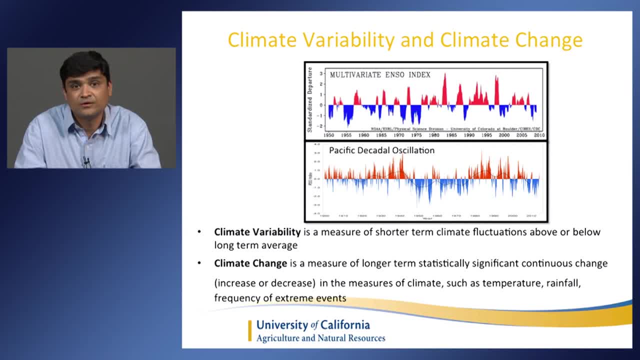 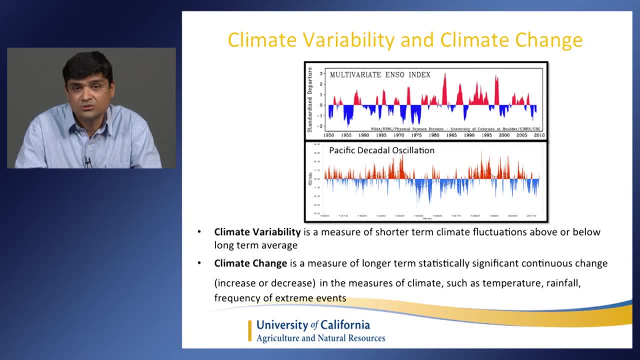 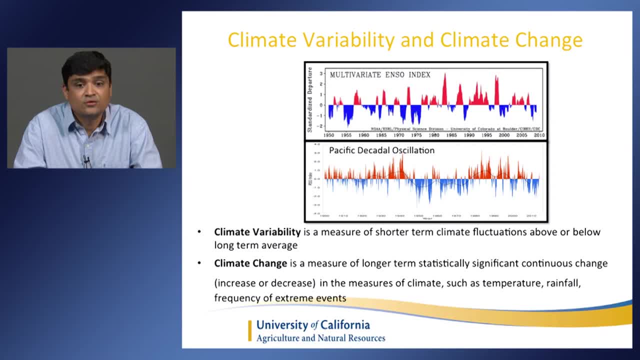 And that's actually a much more pronounced word. absolutely, Yeah, Yeah, Are those things? Absolutely Yeah, We're going to talk about that. So how, those types of things? caniş, caniş, describe climate variability to you. What kind of farm are you referring to? 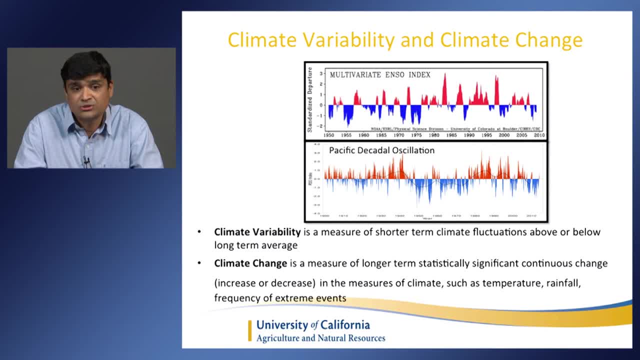 Oh gosh, increases or precipitation or frequency of extremes, or reducing snowpack, extent of snowpack, etc. are some of the examples of climate change. So the major difference between climate variability and climate change is the time frame that we look at in terms of identifying their significant changes. So here is an 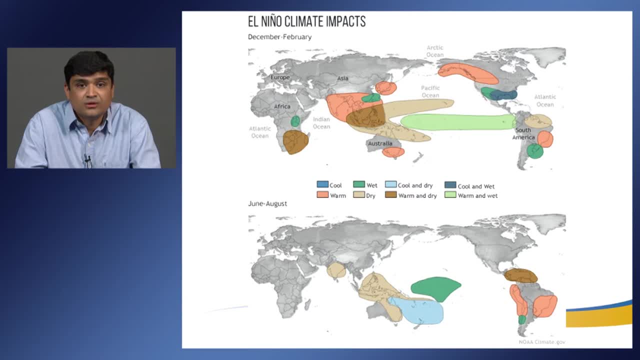 example of how El Nino can impact climate across the globe. The top figure shows climate impacts of El Nino from December through February and, as you can see, their impacts vary quite substantially based on where which location we are looking at. So, for example, in United States during an El Nino. 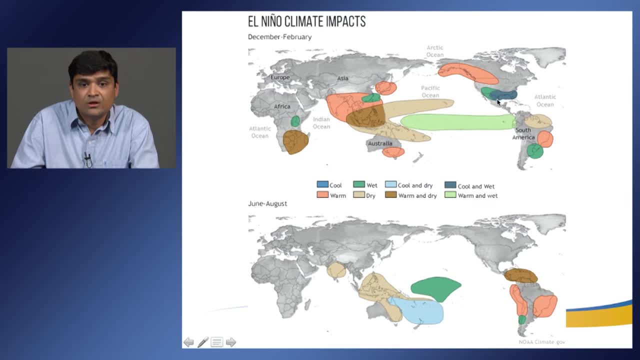 year, during the winter time, December through February, we can expect cooler and wetter conditions in the southern part of the United States, but at the same time, if you look at Asia and most parts of India and in some parts of other parts of Asia, this climate could be. 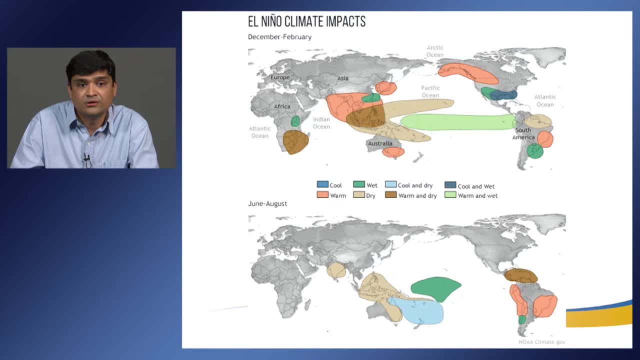 warmer and drier and similar in some parts of Africa as well as in Australia. So depending on which location we are looking at, El Nino impacts can vary substantially. The bottom figure is showing El Nino's impact on climate for during the month of June through August. So, as you can see, there are no signals. 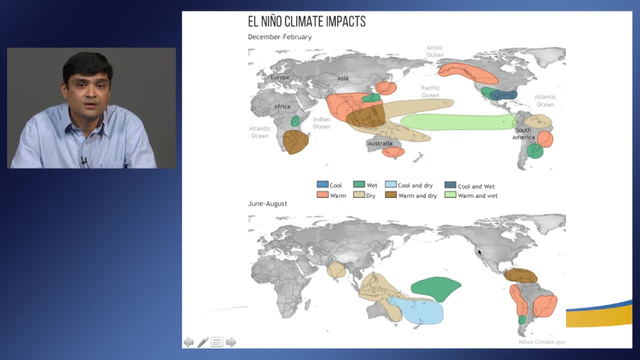 here in United States is because ENSO signals for summer time in United States is very weak and we sometimes don't even get a signals in this area. but if you look at South America during the summer time, you can expect warmer conditions and drier conditions in this area, similar in parts of Asia and India as well. So as 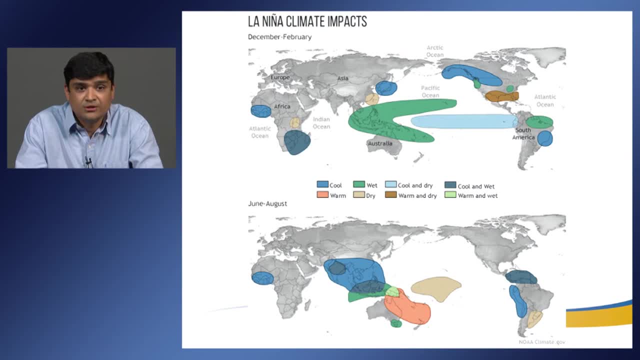 opposed to El Nino conditions during the La Nina phases. during the December to February you can expect a wetter conditions in this area versus warmer and drier conditions for southeast or southern part of the United States, but at the same time you can expect cooler conditions in northwestern. 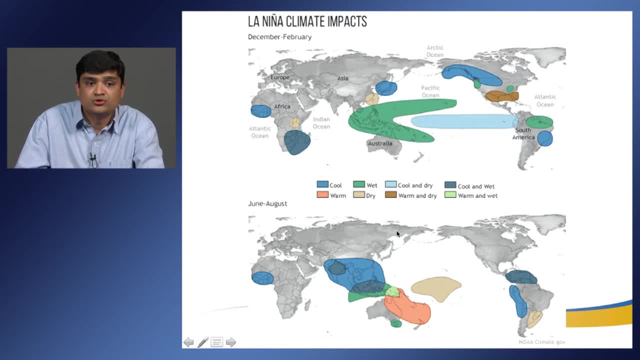 part of the United States. If you move to June through August for La Nina conditions, this area can expect cooler conditions, but parts of Australia is could expect warmer than normal conditions and South America in general this area is cooler and this area is drier. so depending on the location, La 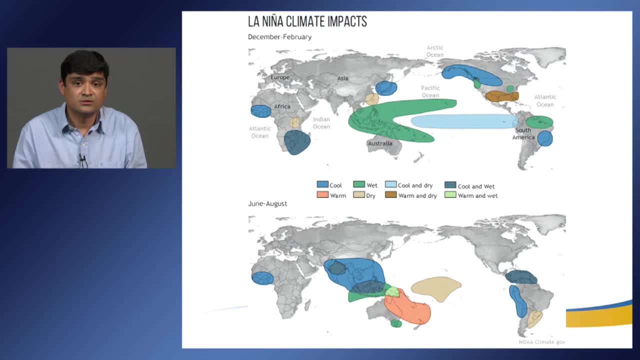 Nina impacts or El Nino impacts could be significantly different If we talk about California. if it is not a strong El Nino or strong La Nina, there are a lot of uncertainties or variability in terms of what we expect in terms of precipitation. So skills in terms of predicting how the water year is going to. 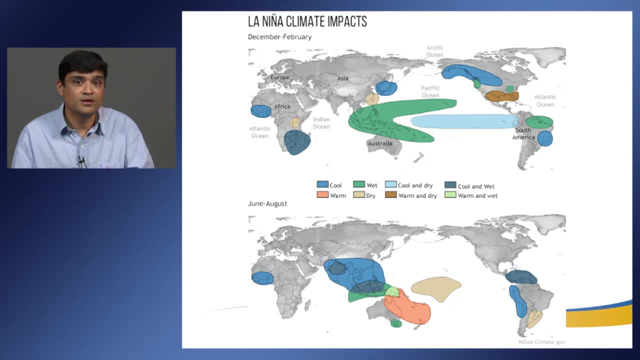 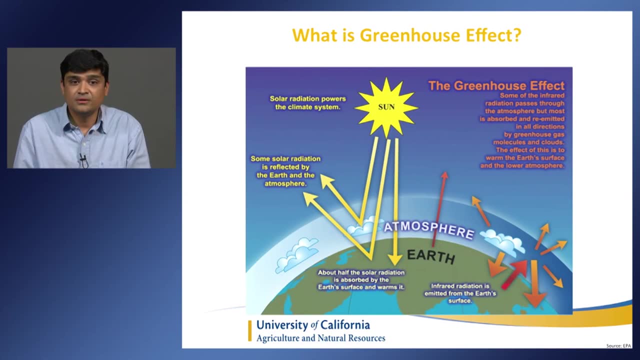 be. If it is a moderate or weak El Nino or La Nina, we might not get pretty reliable skills in terms of predictions. So now let's talk about some of the basics about climate change. As we know that greenhouse gas emissions create warmer, 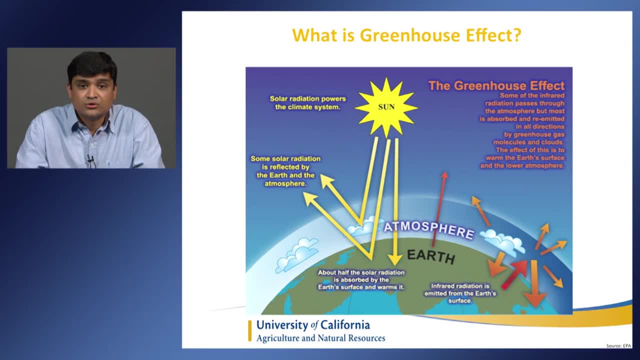 conditions due to the process called greenhouse effect. So in this figure I'm trying to show what the greenhouse effect is. So when the energy from Sun is coming toward the Earth's surface, part of this energy is reflected back into the space, which is no longer a useful energy. But half of this energy is 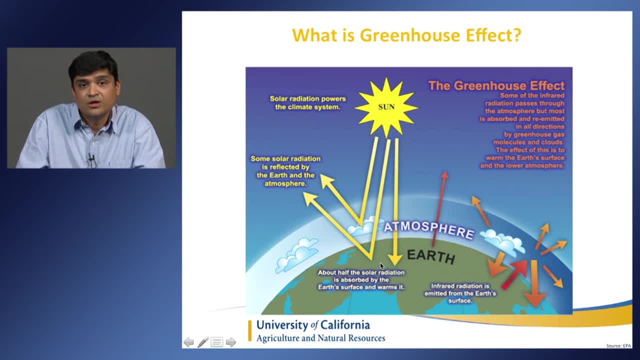 absorbed by the Earth's surface and then Earth re-emits that energy in terms of infrared radiation or longer wavelength radiation, And this greenhouse gas emission is a very important part of climate change. So if we look at the atmosphere, we can see that greenhouse gases have a tendency to absorb this. 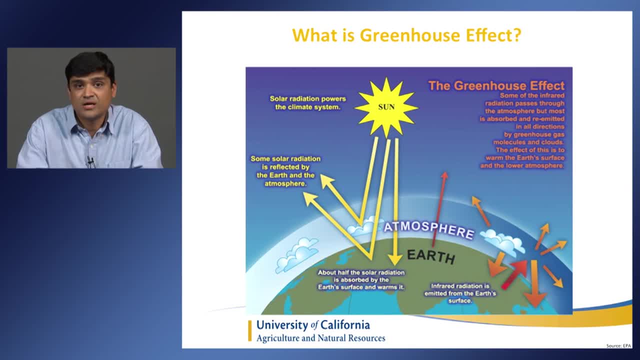 longer wavelength radiation and then re-emitting to all these different directions through the process called scattering. So when you have higher concentration of greenhouse gases into atmosphere it sort of traps this energy and warms the globe And the whole process is called greenhouse effect. And 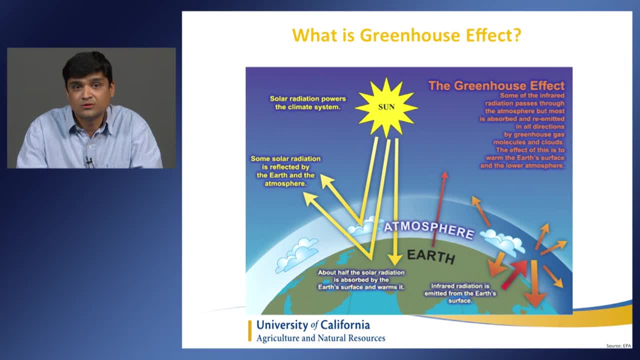 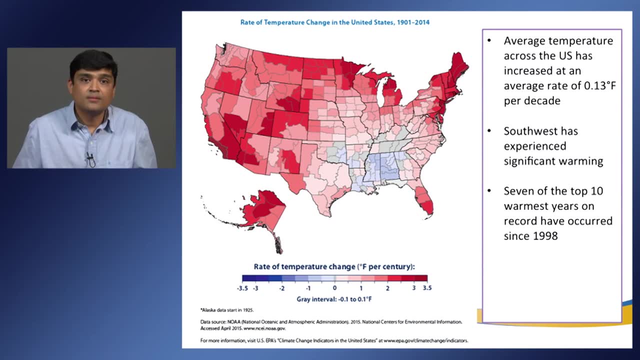 due to this increase in the greenhouse gases and due to the interaction of other parameters, we can expect significant changes in the climate. So let's talk about some of the indicators, about what we have experienced so far. in the last hundred years or so, This figure shows rate of temperature changes in the 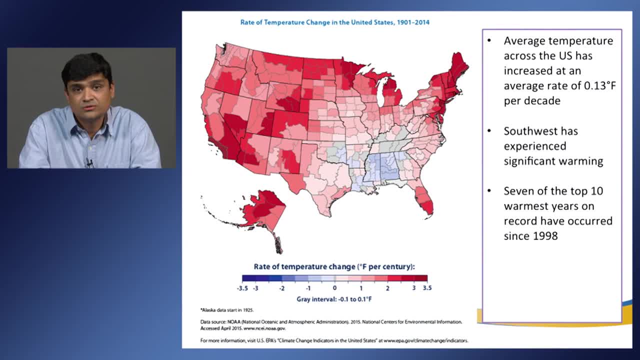 United States from 1901 to 2014.. And this is comparing with climate normals, which is from 1980 to 2010.. Again, an average temperature across the US has increased at the rate of 0.13 degrees. 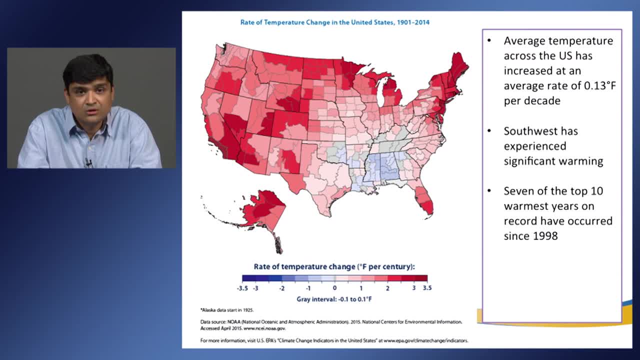 Fahrenheit per decade And, as you can see, southwestern part of the United States did experience substantial warming in the last 100 years- anywhere from 2 to 3.5 degrees Fahrenheit for 100 years period. But at the same time some parts of the southeast part of the United States did experience somewhat. 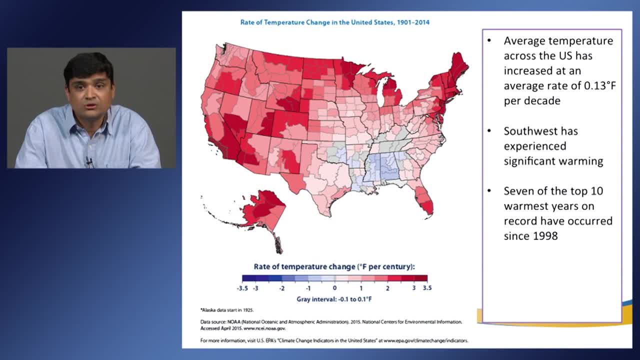 cooling effect. But overall, in general we did have increase for the entire United States, And that is similar for global conditions as well- And seven out of top 10 warmest years on record have occurred since 1998.. So in the recent years this warming has been substantial. 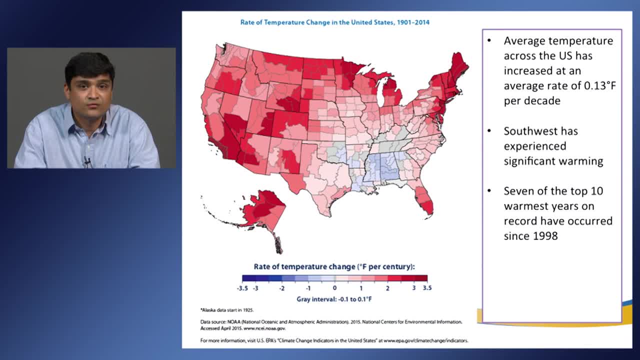 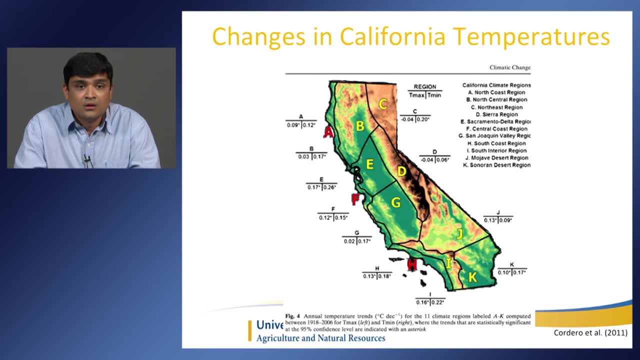 Actually higher as it was used to be. in 2014 year was the warmest year on record as well, globally. If we focus on California, this figure shows rate of temperature increases both in maximum and minimum. So if you look at all these different climate zones, this represents T-max and this represents. 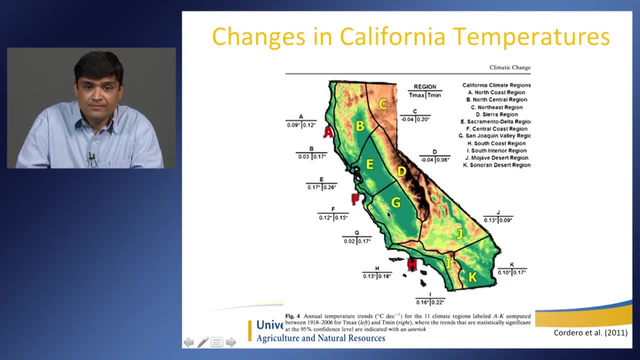 T-min And, as you can see, for example, San Joaquin Valley, which is heavily agricultural area, there is not a significant increase in terms of maximum temperatures, But if you look at the rate at which minimum temperatures have increased is substantially. 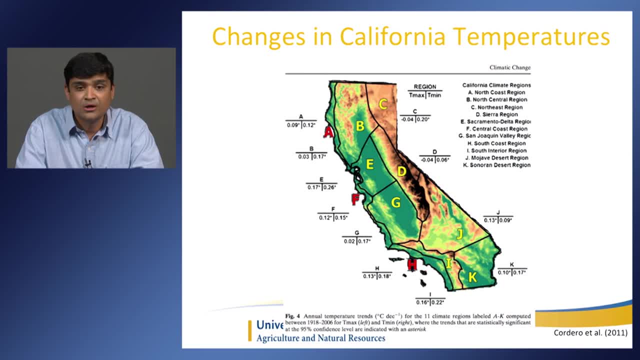 higher, And it's a similar trend for almost entire California, All these different zones. that rate at which minimum temperatures are increasing are substantially higher than the rate at which maximum temperatures are increasing And this, specifically, can have a significant impact on agriculture. One is that with this rate of increases you might have more rate of respiration and that 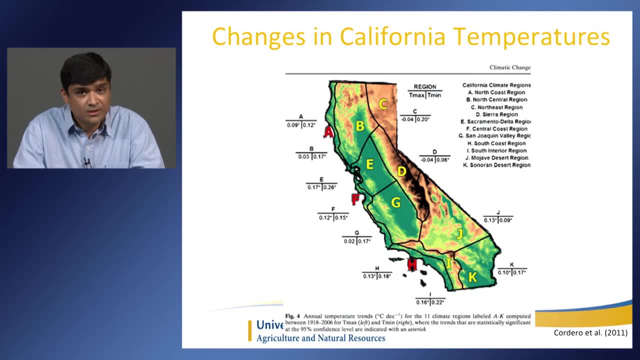 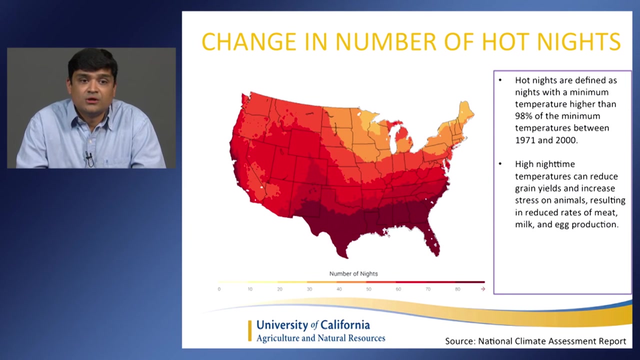 can adversely impact yield. Another consequence would be lower accumulation of chill hours, which is very significant for many of the net crops. 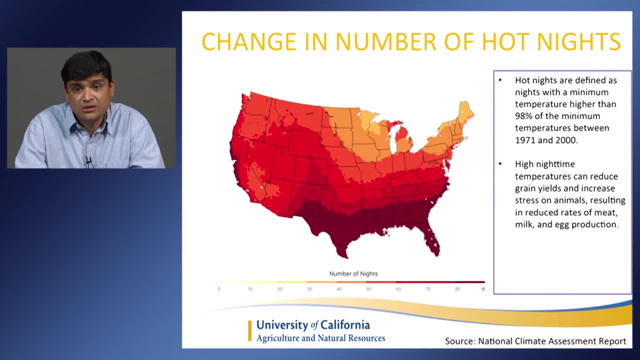 as night, with the minimum temperatures higher than 98 percent of the minimum temperatures between 1971 to 2000.. So high nighttime temperatures and, as you can see from this figure, southern part of the United States and some parts of California have significantly higher number of nights. 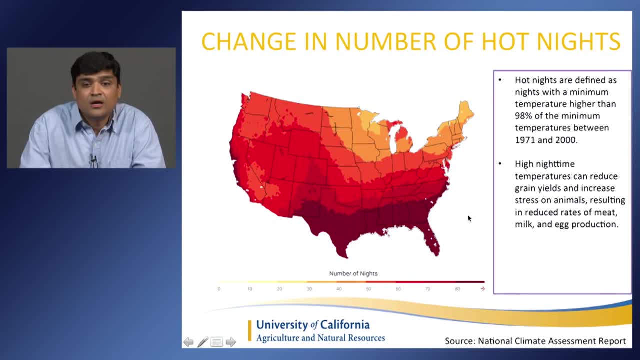 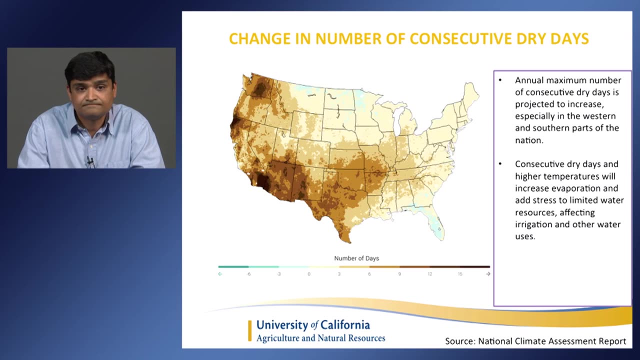 compared to other parts of the United States, And with the high nighttime temperature, it can reduce grain yields and increase stress on animals, resulting in reduced rate of meat, milk and egg production, along with reduced crop productions. This is another slide that I pulled from National Climate Assessment Report. is changes in number. 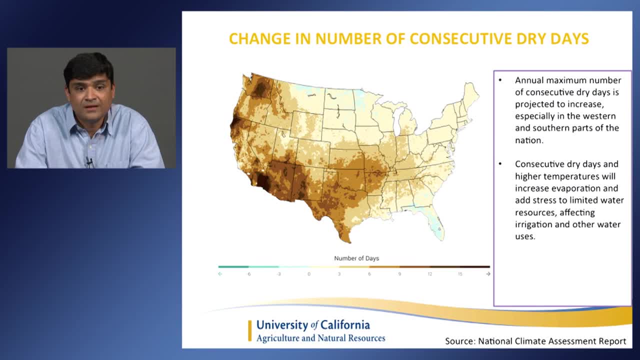 of consecutive dry days And, as you can see, southwest in general has more number of consecutive dry days compared to the other parts of the United States. Annual maximum number of consecutive dry days is projected to increase, especially in the western and southern part of the United States. 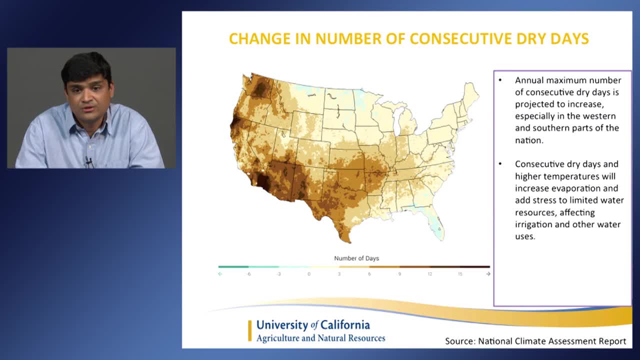 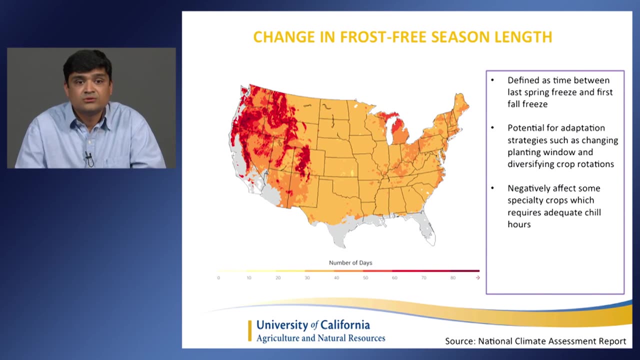 Consecutive dry days and higher temperatures will increase evaporation and stress to limited water resources, which is one of the significant impact of climate change for California as well, affecting irrigation and other water uses. Changes in frost free season length, so the frost free means the duration between last 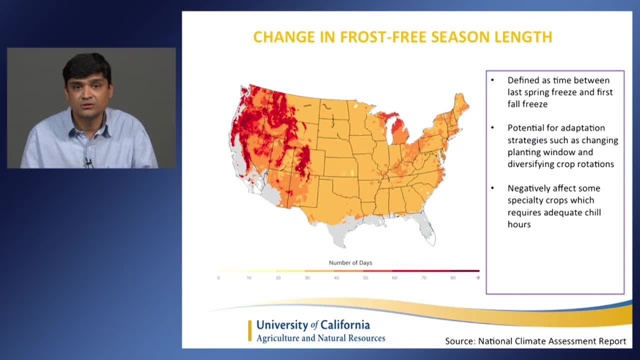 spring freeze and first fall freeze, So that duration has been increasing across the United States and especially on the western half of the United States that number of frost free dates are substantially higher than the other, than the eastern part of the United States. 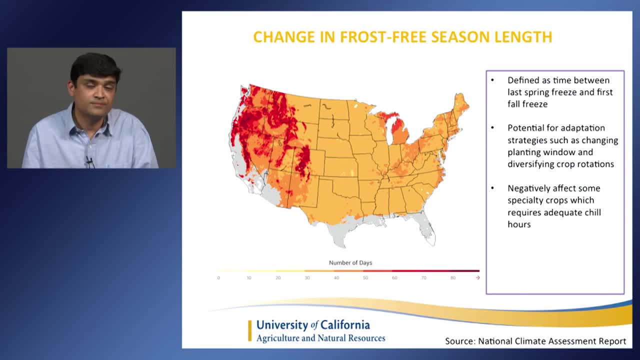 And that can also have a positive impact In terms of adaptation. for example, if you are looking at an annual cropping system, you can adapt or change the planting dates and change the cropping pattern with respect to this frost free season, so you can have a longer growing season. 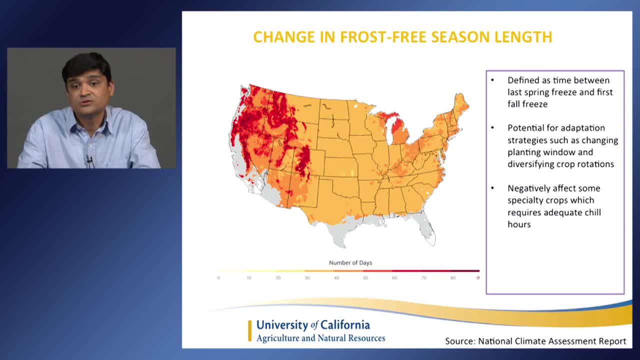 On the other side, for perennial systems, it can negatively impact because some of the specialty crops require adequate chill hours And, with this trend, it can also have a negative impact. because some of the specialty crops require adequate chill hours. It might be negatively impacting the frost in terms of their getting enough chill hours. 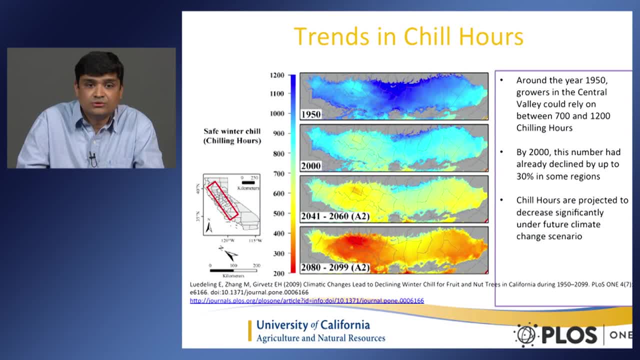 Here is the trend in chill hours. This is a sketch for Central Valley in California And if you look at 1950, growers in around 1950, growers in Central Valley could rely on between 700 to 1200 chill hours. And if you look at the 1950s growers, in around 1950, growers in Central Valley could rely on between 700 to 1200 chill hours By 2000,. that number has reduced by 30% already. So that's a significant reduction in number of chill hours accumulated for California. 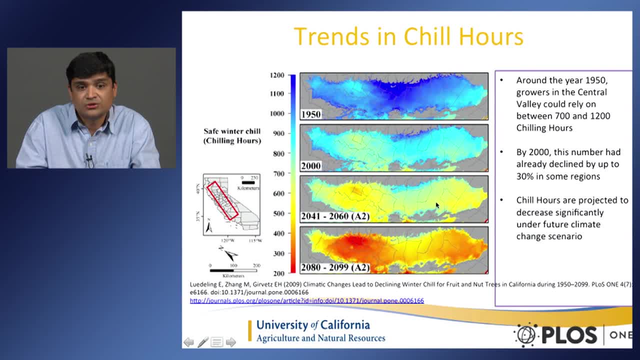 And under future projections or high emission scenarios, chill hours are projected to decrease significantly, and that could be ranging anywhere from 200 to 400 by 2080 to 2090, and 400 by 2070 to 700 from 2041 to 2060. 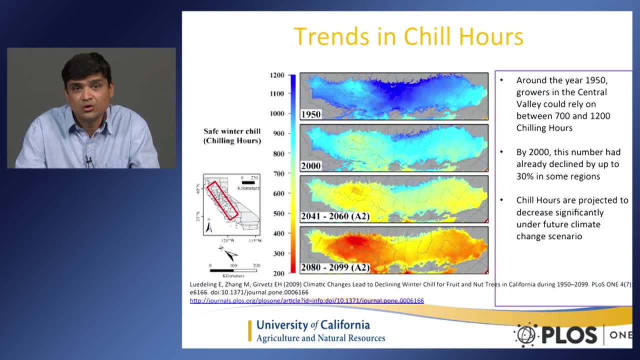 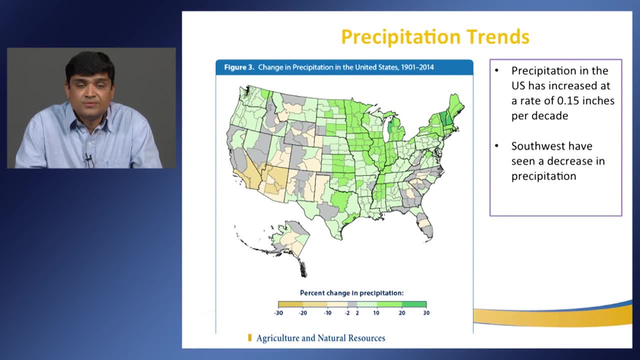 So we could expect significantly lower number of chill hours in future climate projections. Here is the precipitation trend with respect to last 100 years. So if you look at last 100 years, overall for United States rate of precipitation has increased at the rate of 0.15 inches per decade. So overall we have a lot of precipitation. So if you look at last 100 years, overall for United States rate of precipitation has increased at the rate of 0.15 inches per decade. So overall we have a lot of precipitation. 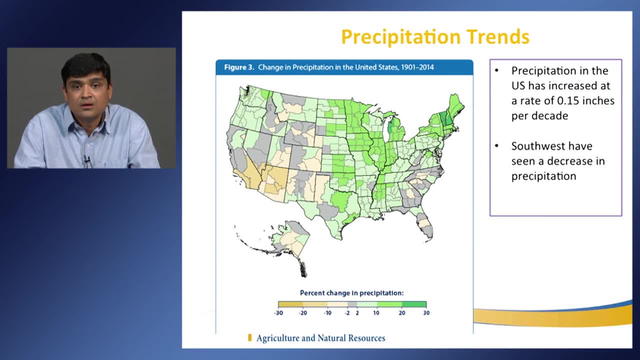 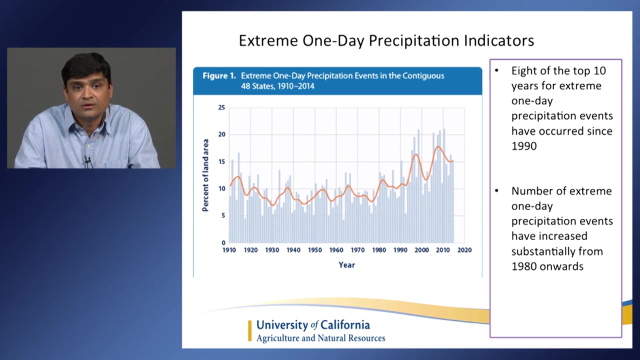 We have seen wetter than normal conditions, But on the other side, southwest has seen decrease in the rate of precipitation for last 100 years, So even with those areas where we did experience wetter than normal conditions. at the same time, we are also seeing increase in number of single-day precipitation events. 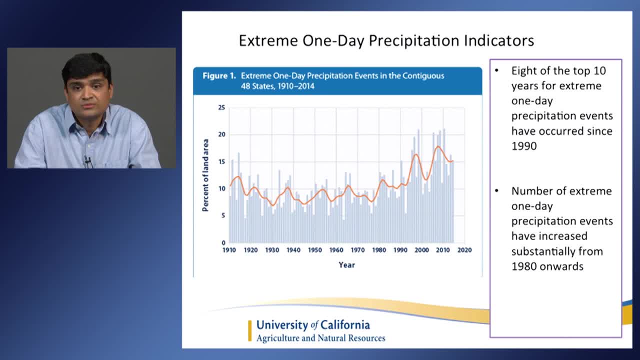 So eight out of 10 years of extreme single day precipitation events has occurred since 1990.. So in the recent years this extreme single day precipitation events has been occurring quite often, as used to be in the past. Number of extreme single day precipitation events. 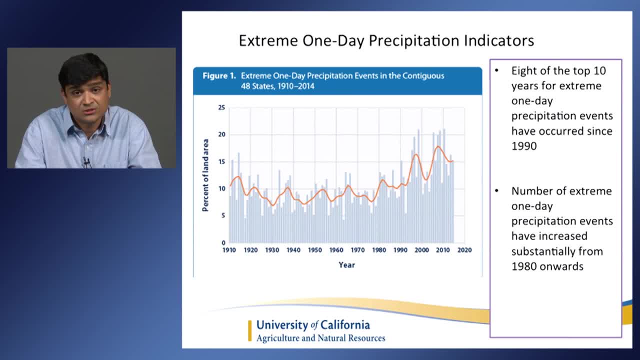 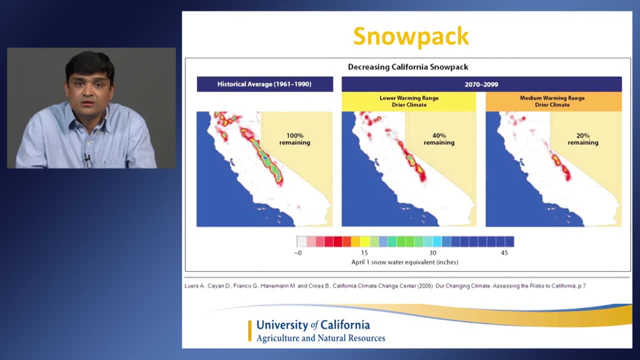 in general from 1980 onwards has increased substantially And that could also have adverse impact on agriculture. Snowpack is our natural water storage for California. In terms of so far, we have seen approximately 10% reduction in the snowpack for California. 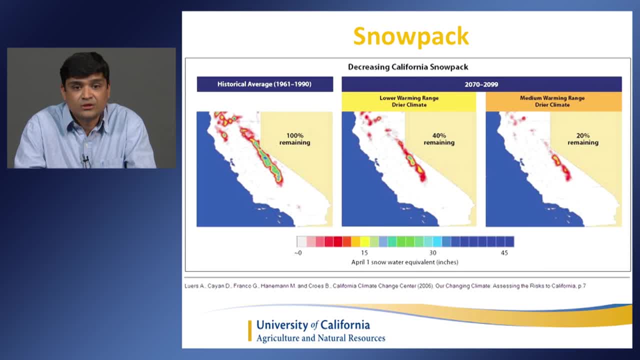 And under low emission scenario we could expect 40% of remaining snowpack And in a medium warming range or medium climate scenarios that could result in 20% remaining snowpack. So by 2070 to 2099 during that timeframe. 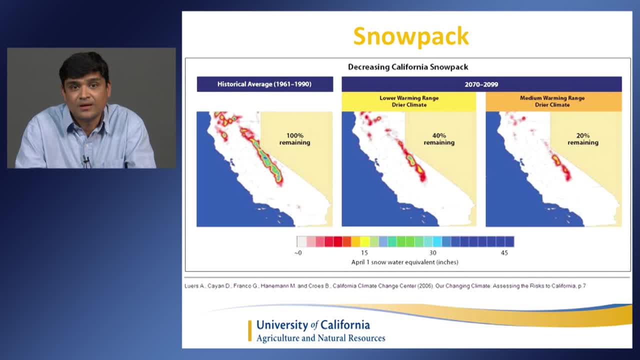 So that's a substantial lower snowpack that we could expect in a future climate change projections. According to the scientist, we can also expect 25% reduction in snowpack by 2050.. So all these models are showing decreasing trends in the snowpack. 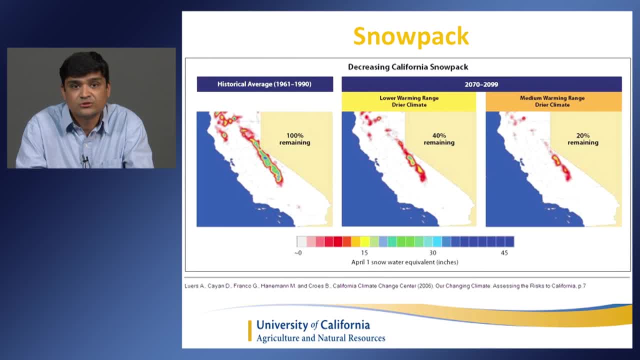 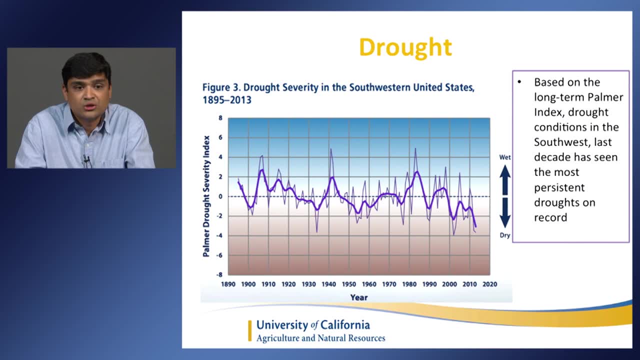 which could adversely impact the total water supply for the state. In terms of drought, this particular figure shows a time series of Palmer Drought Severity Index And, based on that particular index, last decade has been persistent drought for the Southwestern part of the United States in general. 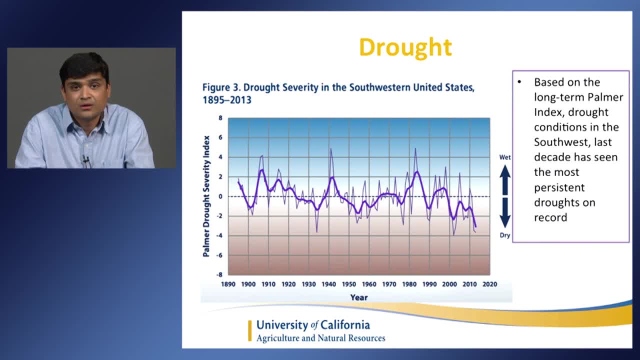 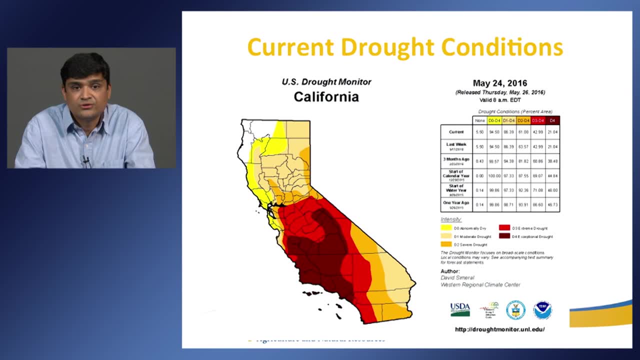 And we could expect to see more of this frequent drought conditions in the future climate change projections as well. Here is the current drought conditions. Since we had one of the strongest El Nino on record, it did provide some relief to five years drought conditions. 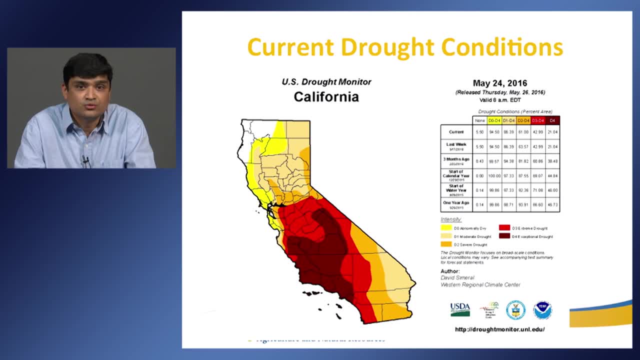 that we had, but it was not even enough to completely get the drought out of California And we are still. many parts of especially the Southern part of the California is under exceptional drought conditions And most of the other part of California are still in moderate 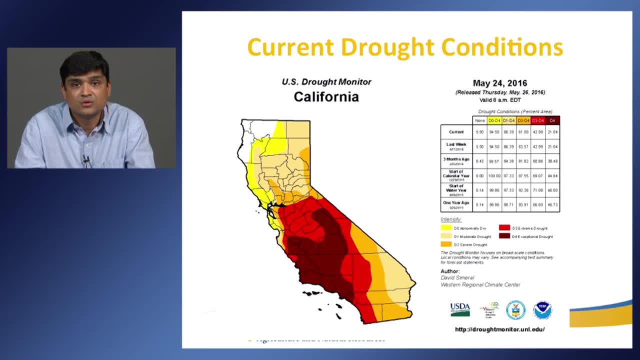 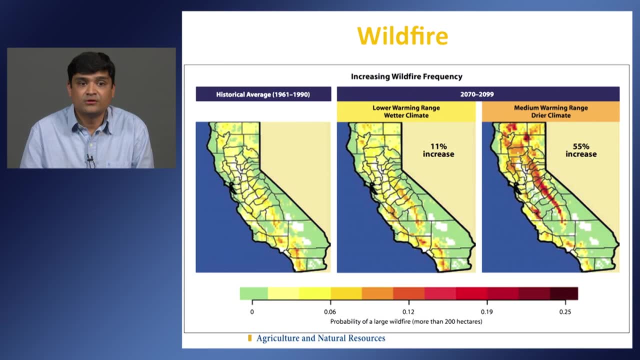 to severe drought conditions as well. So this is the current drought situation In terms of wildfire, if you compare it with the historic average from 1960 to 1999,. under low warming range, risk of wildfire can increase by 11%. 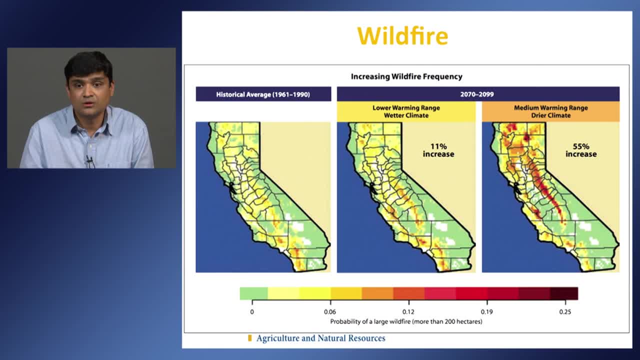 And the same risk under medium warming range could increase up to 55% And the same risk under medium warming range could increase up to 55% And the same risk under medium warming range could increase up to 55% And that could be a significant economic impact for the state. 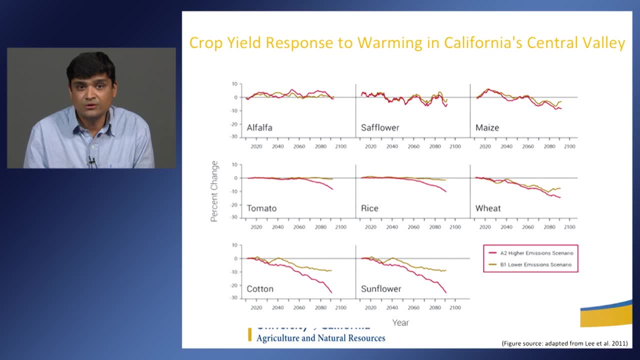 This is a result from a modeling study where they looked at crop yield responses to warming in California Central Valley. In this particular modeling study they looked at they kept the water as an adequate level So there was no water stress in this condition. 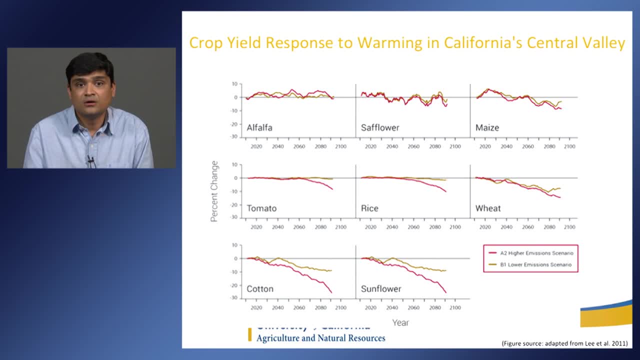